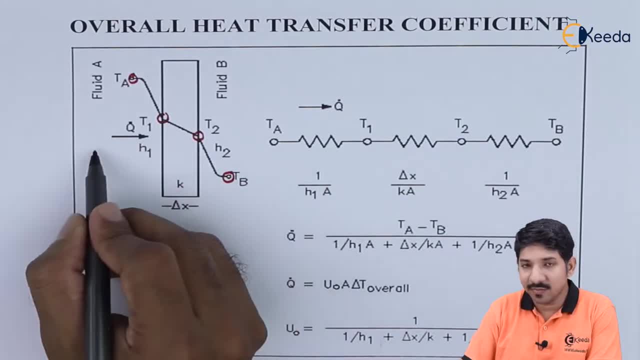 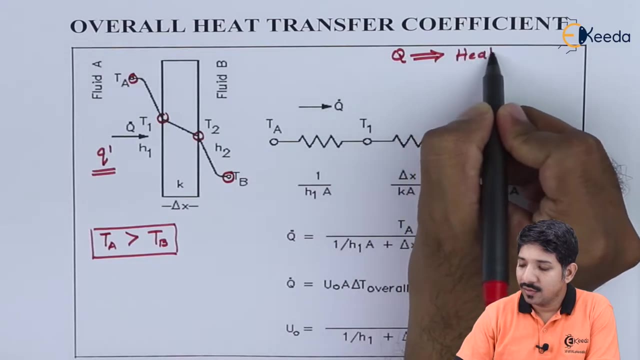 So if this is the case, obviously the heat will get transferred from the left to right. So let us call that heat as Q' I have told before that this capital Q is nothing but the heat. Now this talks about the amount of heat. 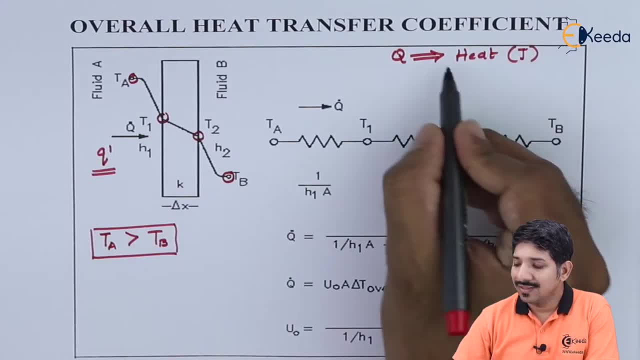 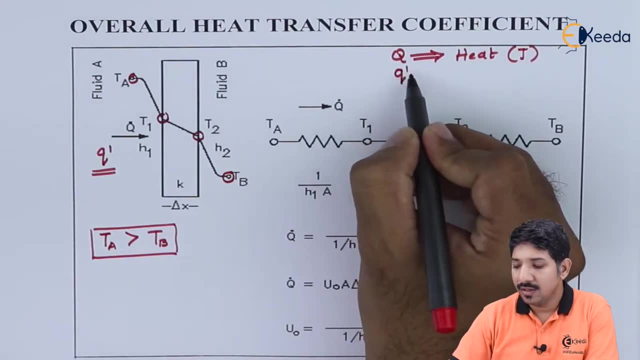 The unit for the same is joule. Now, this is what we have studied in the thermodynamics. Now, when we go to the heat transfer, this should be replaced by the Q' Now this Q' talks about the rate of heat transfer. 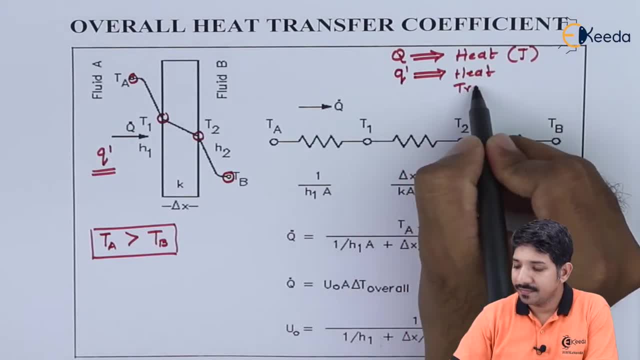 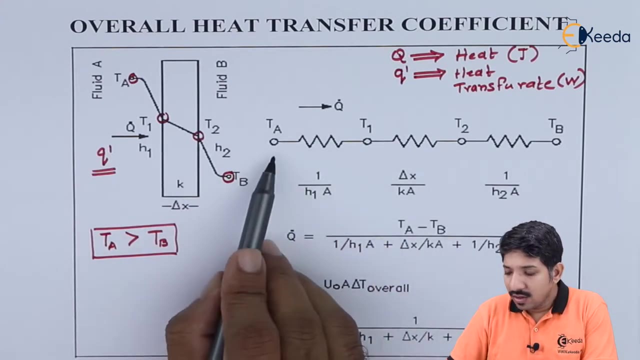 Or the heat transfer rate. The unit for the same is obviously joule per second, that is Watt. So just to have this differentiation, we will not use capital Q, We will use a small Q' Now if I want to draw or if I want to show the thermal circuit diagram for the same. 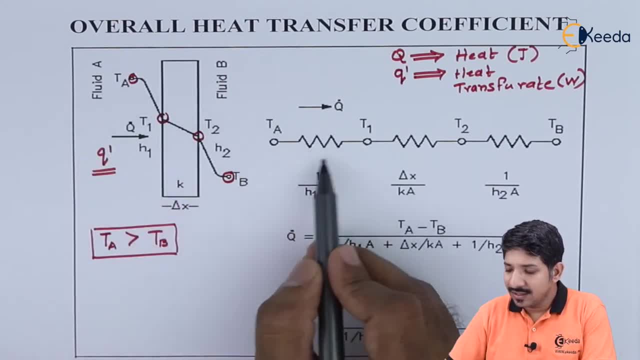 this will look something like this TA, that is, this temperature, Then the thermal resistance. Now, this resistance is nothing but the resistance offered by the. Now, this resistance is nothing but the resistance offered by the. Now, this resistance is nothing but the resistance offered by the. 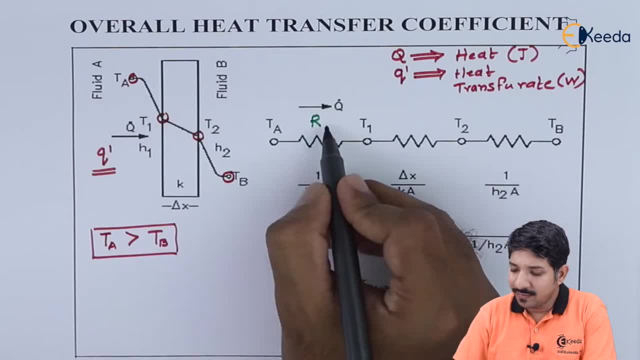 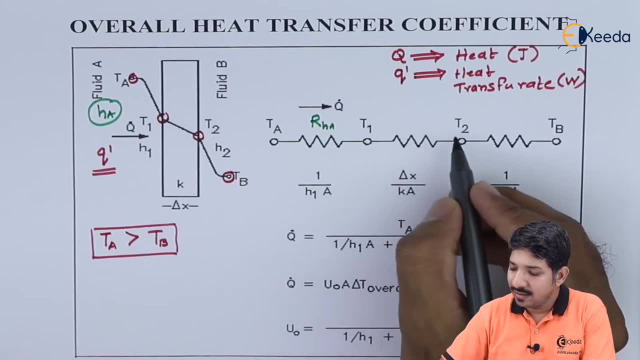 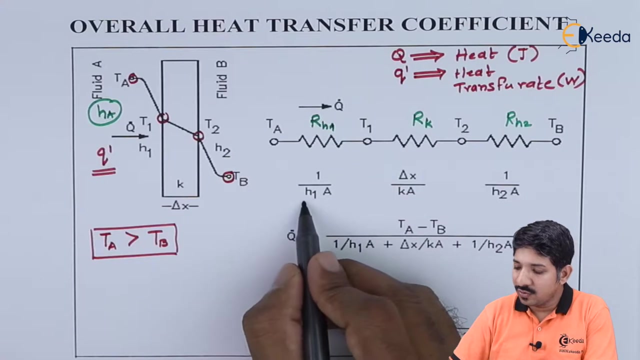 fluid A. So let me call RHA, where HA stands for heat transfer coefficient for the A side. Similarly, this is your thermal resistance offered by the conduction. Let us say RK, and this is, let us say, RH2.. So let us call H1 itself, because we have used H1 in the denominator. 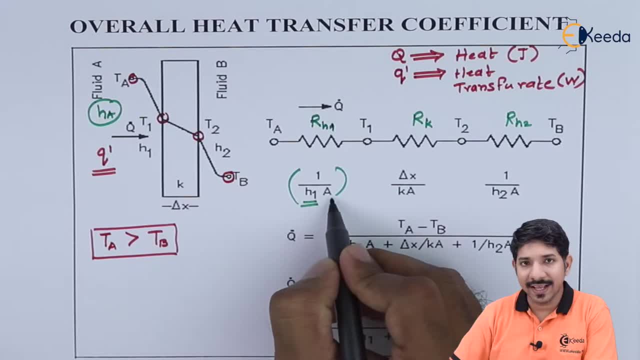 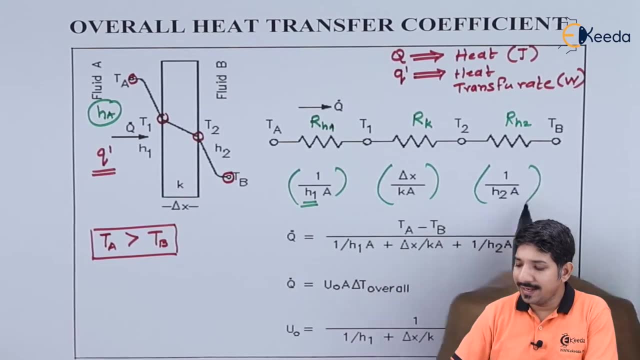 So the thermal resistance is obviously 1 upon H1A. Here this is L upon KA. In this case my L is delta X. So delta X upon KA, and here we have got 1 upon H2A. So this thing we have done before. 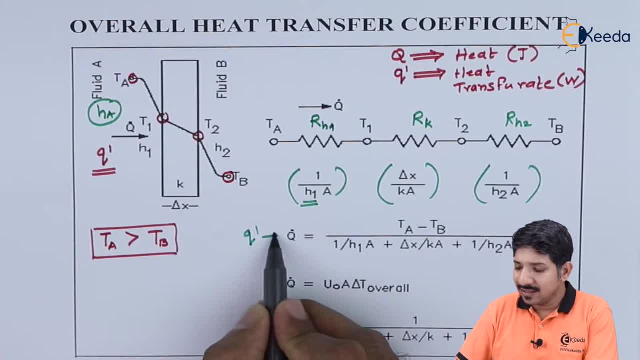 So if I want to write down the value of Q', it can be written as TA minus TB, That is, to extreme temperature divided by all the thermal resistance. Now this can also be indicated as: Q' is equal to UA delta T. 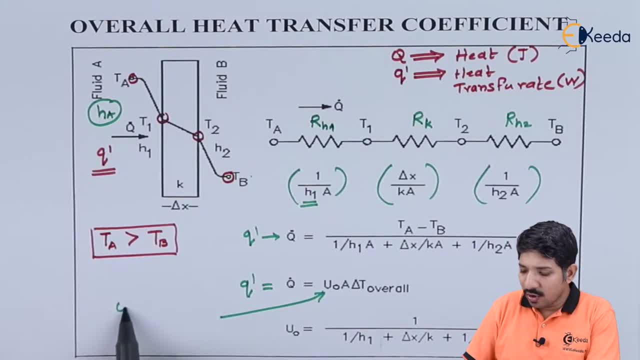 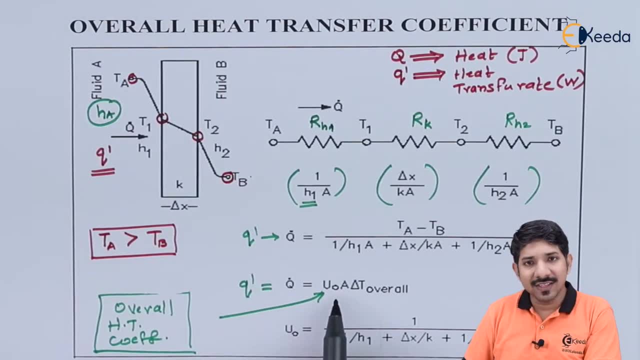 Now here this? u is called as the overall heat transfer coefficient. Now, what is the significance of this? we will see it later, but first of all, for this case, my value of u will become something like this here: what we have done, we have taken this a common and if 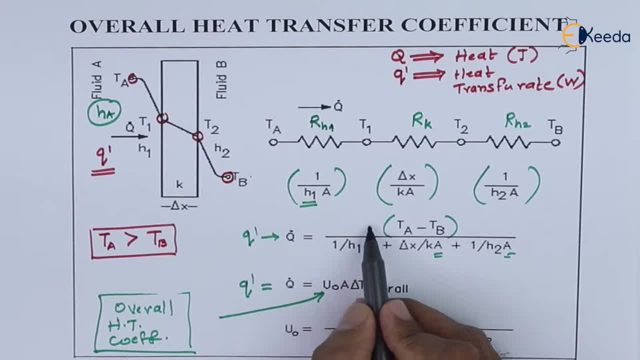 I take it to the other side, so I will have a somewhere here and this is my delta t. so a into delta t. so whatever is left over here is must be u So u or u naught is what we have said over here. this u naught is equal to 1 upon h a plus delta x upon k plus 1 upon h 2.. Now this in the inverse: 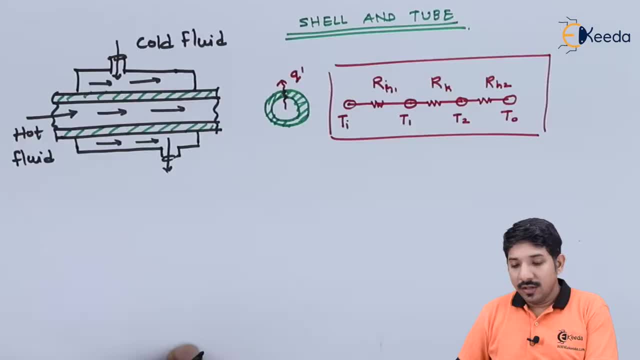 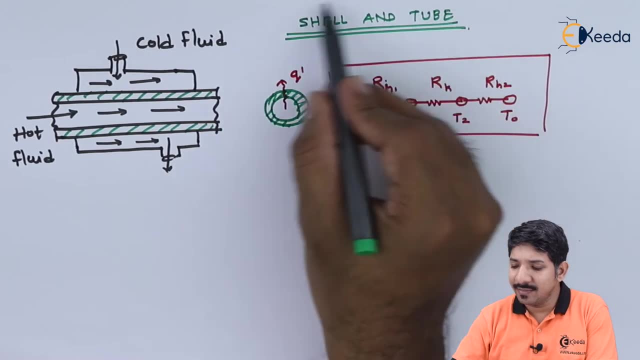 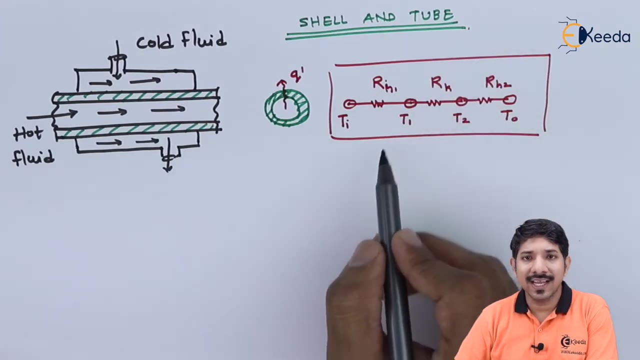 ratio is nothing but your overall heat transfer coefficient. Now, previously we talked about a simple wall and fluid arrangement. Now the same thing can be said about the shell and tube heat exchanger. So let us talk about the overall heat transfer coefficient for the shell and tube type of heat exchanger. So again, let us consider: this is the 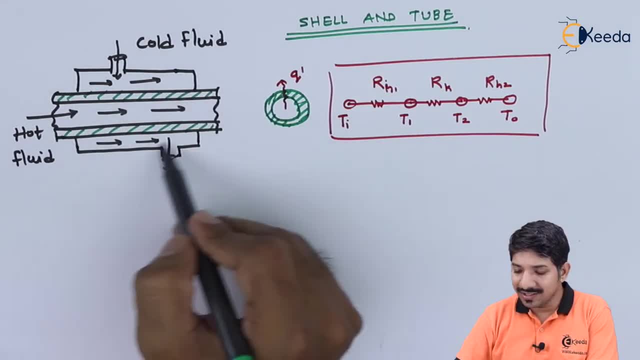 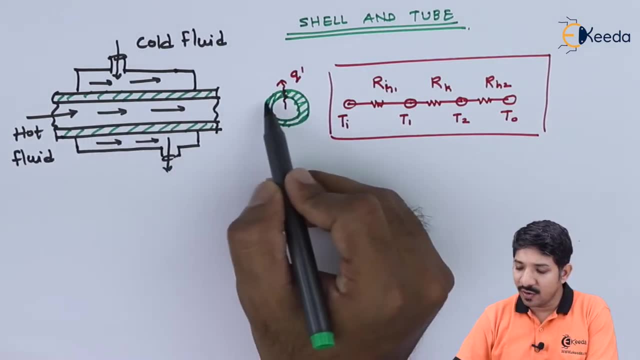 small section of a shell and tube type heat exchanger where from the shell we have a cold fluid and from the tube we have a hot fluid. If this is the case, then if the heat is flowing from the hot fluid to the cold fluid, then we can draw this kind of a thermal circuit diagram. 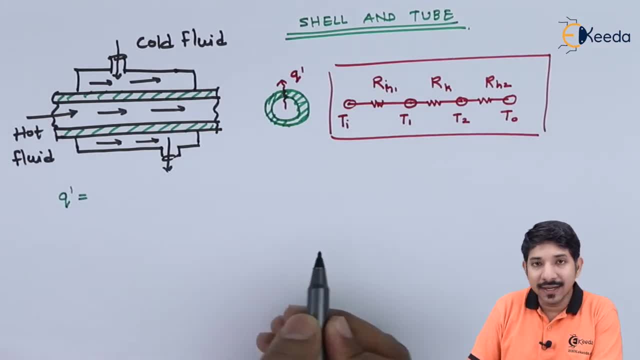 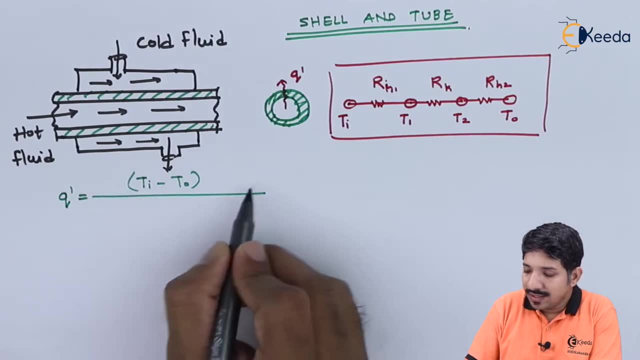 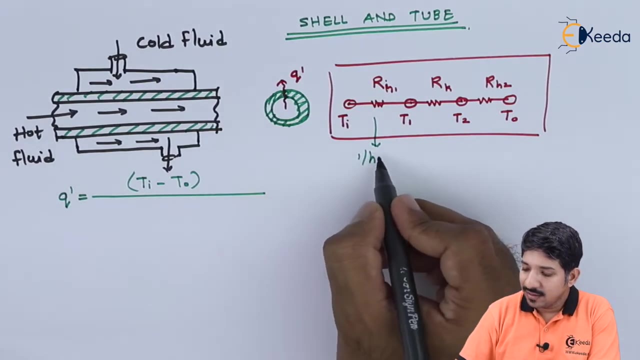 So in this case again, I can write down this q dash can be written as the delta t, that is t i minus t o divided by all the thermal resistance. Now, obviously this one is 1 upon, let us say h, 1 a. this one, Now, this is a. 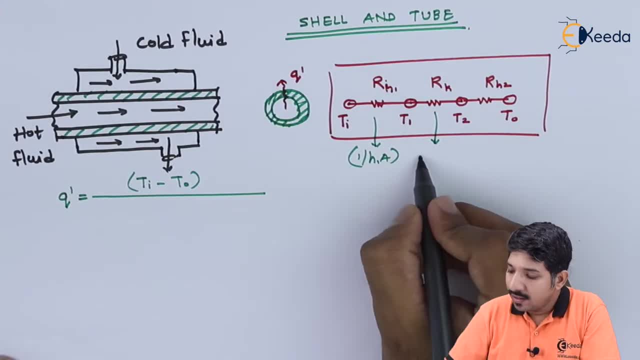 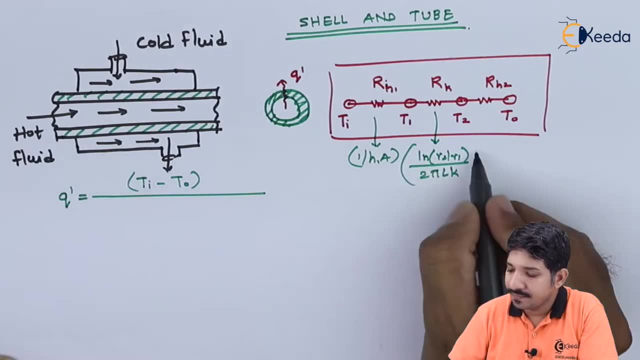 circle. Now for the circle, we know. this is given as ln of r 2 by r, 1 upon 2, pi l k. Similarly, this one is again given as 1 upon h 2 into a. Now, in this case, you need to understand. 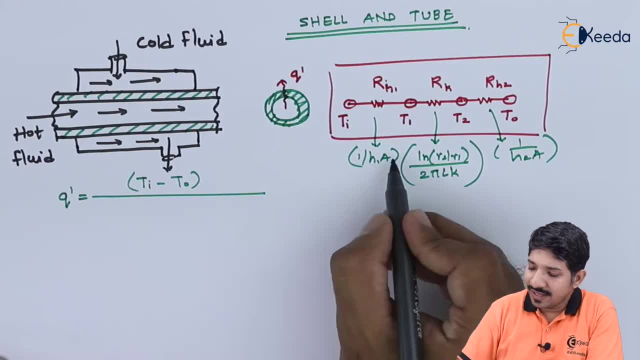 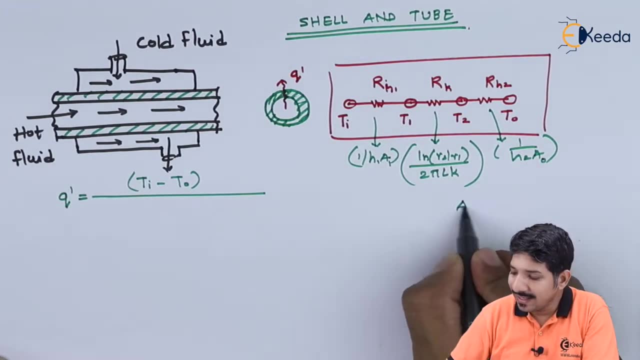 that we can simply write this over here. where we can write this a? Now, in this case, my area is the inner area and here my area is the outer area. What is my inner area? it is 2 pi r 1 into l2, divided by 2 pi r 1 into a l2.. 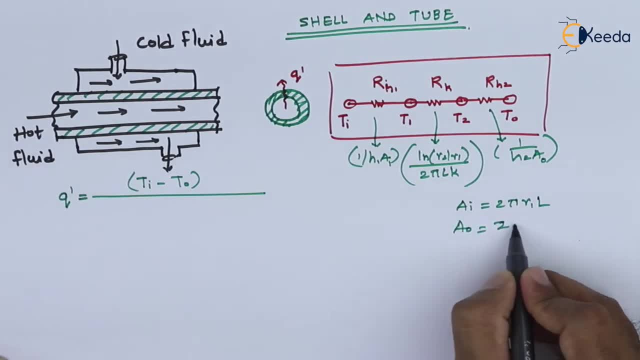 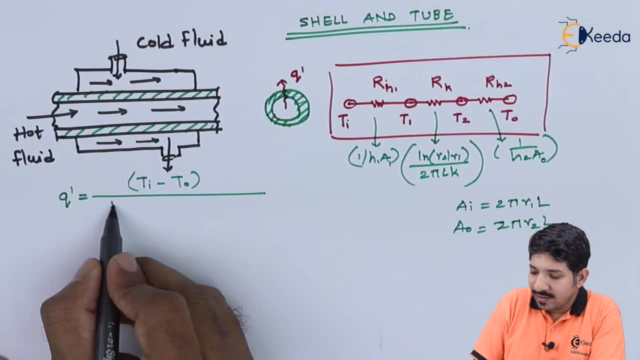 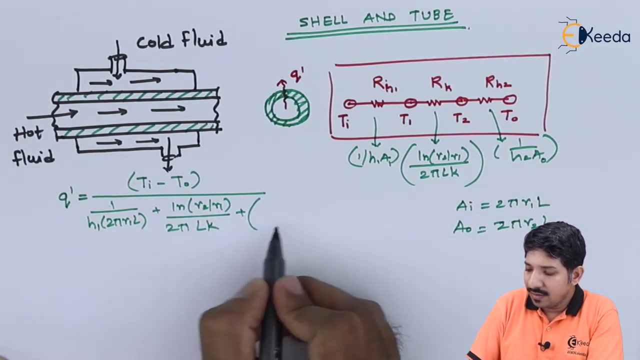 and AO is 2 pi R2 into L, So let us substitute the same thing over here, So this will become 1 upon h1, and here we got 2 pi R1 into L plus ln of R2 by R1 upon 2 pi Lk plus 1 upon h2. 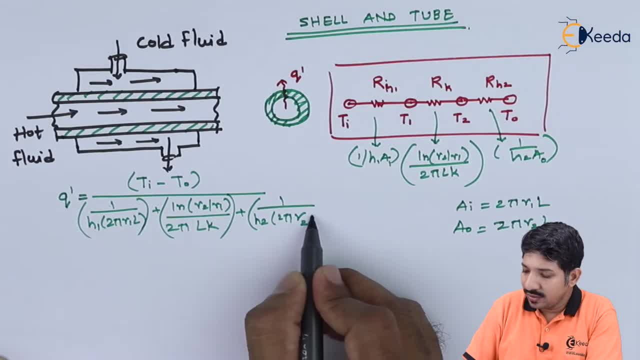 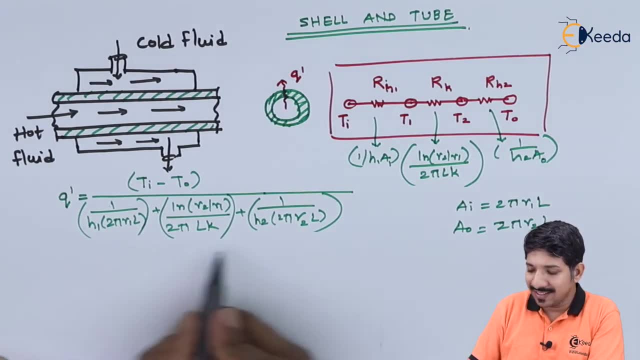 2 pi. Now this is R2 into L. So now again, if I want to simplify it, see, basically we need to equate the same equation with the. this kind of equation, that is, q dash, is equal to UA delta t, where my delta t will be ti minus to. 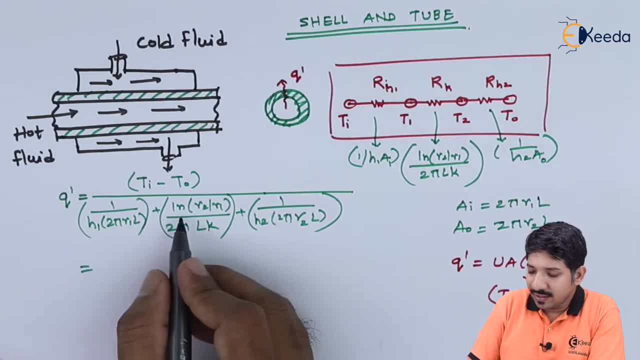 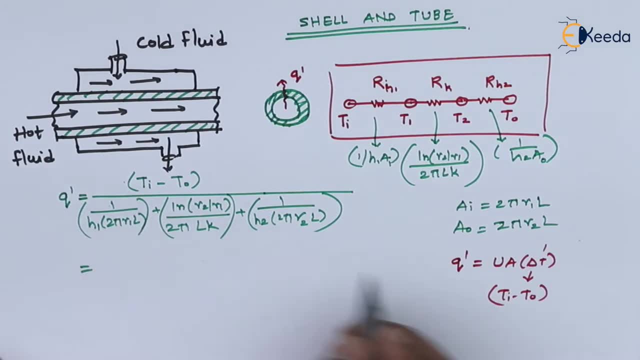 So let us do the further calculation. if I do it, what will I have? I want the area to be at the upper side, So let us take out the area. So if I write down this ai, that is the inner area, so corresponding to this inner area, my ui will be what? so let us take 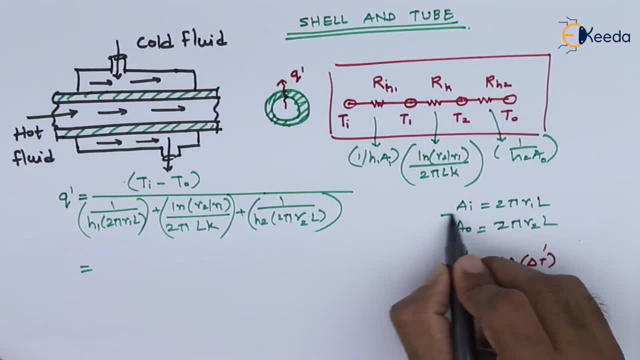 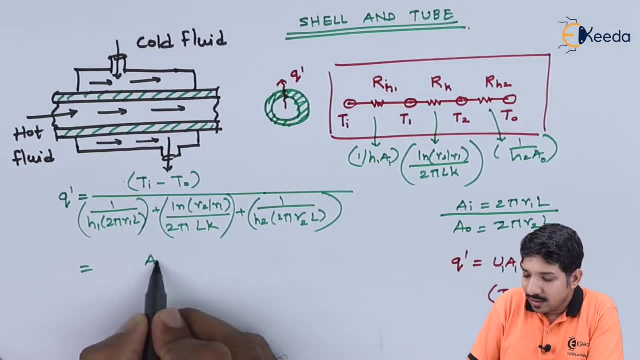 out ai over here. that is 2 pi R1 into L, So let us multiply everywhere. so we have got this as ai. What is this? 0.. into this is my delta d. this I have written as delta d in the denominator of what I am left with. 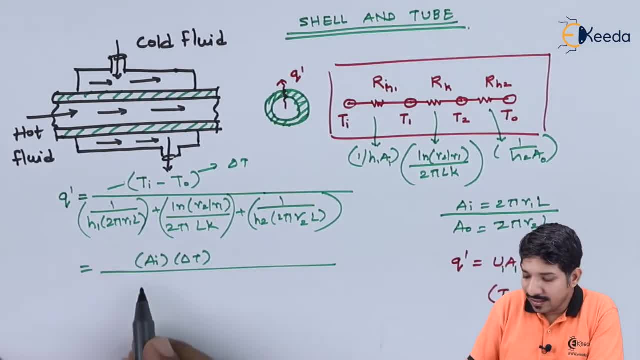 So here, if I multiply everywhere by 2 pi r1 into l, I can write this term as same as 1 upon h1 plus 2 pi lk. So 2 pi will get cancelled out. So we are only left with r1 ln of r2 upon r1. 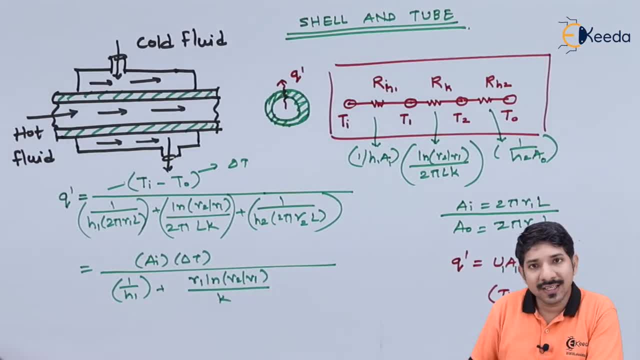 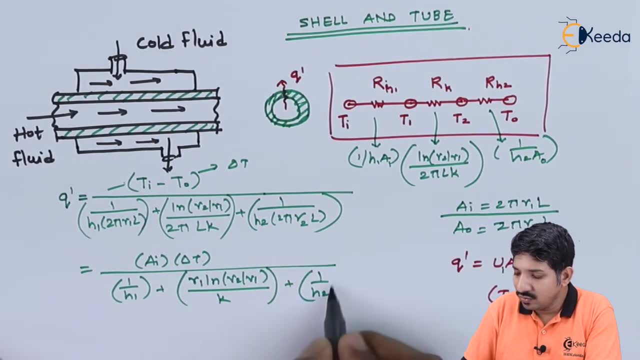 upon, we will have only thermal conductivity k over here, plus here also we can write this as 1 upon h2 and we will end up with the getting a ratio of r1 by r2.. So this way we can find the value of u of i. So this is basically your u of i value the inverse of. 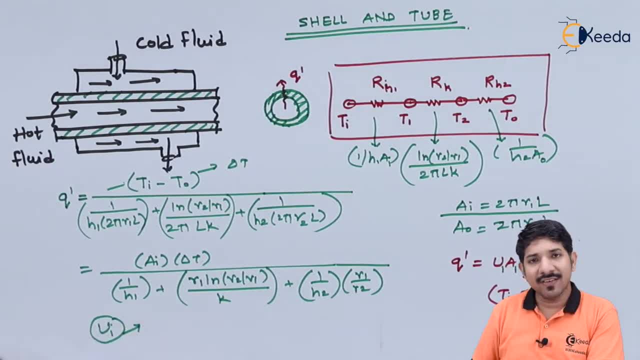 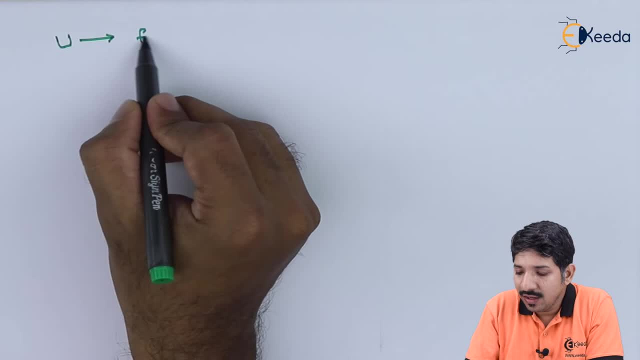 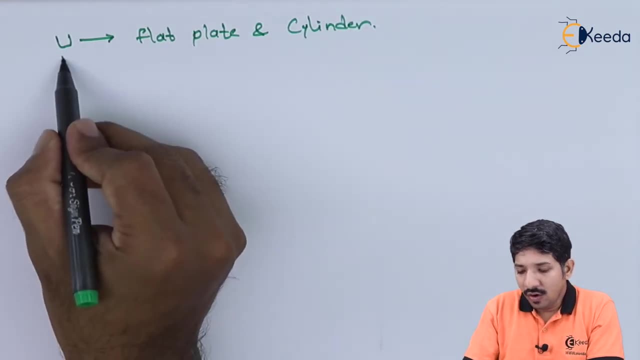 this quantity. Similarly, you can find the value of u of o. So here, basically, we have found out the overall heat transfer coefficient for the flat plate and for cylinder. So we know the value of heat transfer coefficient can be easily found out. So what is the significance of the same? 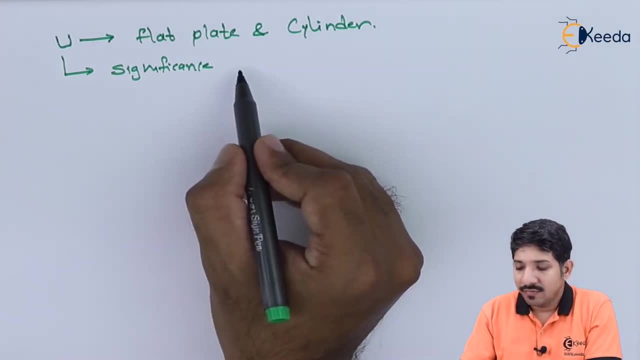 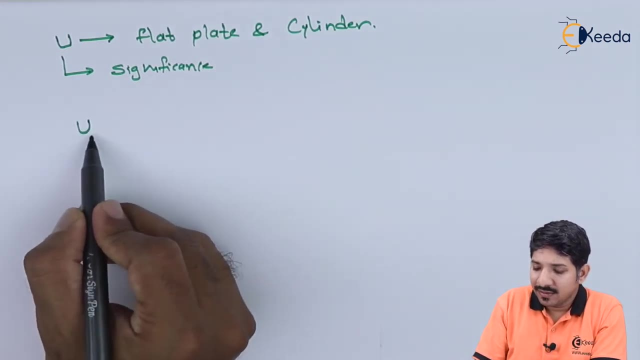 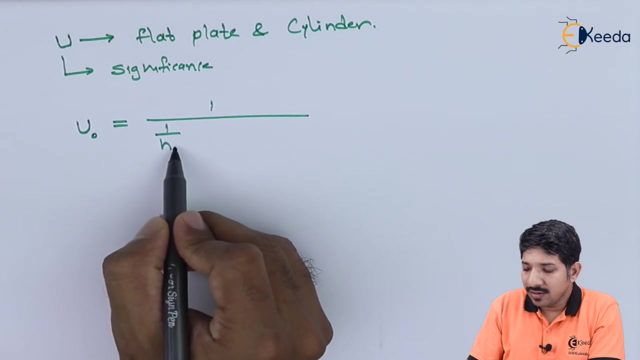 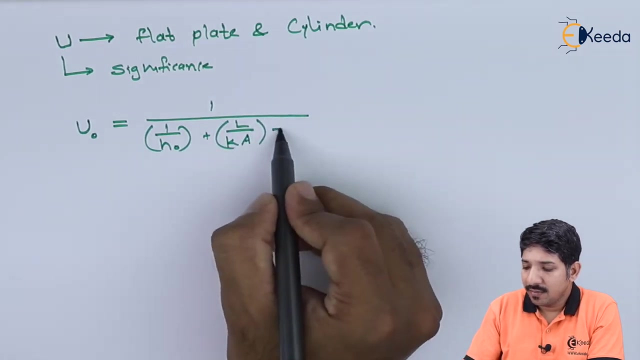 So let us look at the significance of the same from the heat transfer application point of view. So let us consider the flat plate. So for the flat plate, so let me write this: u? o, the value of u? o was 1 upon h? o plus l upon k a, or l upon k plus 1 upon h? i. So now here, in this case, if 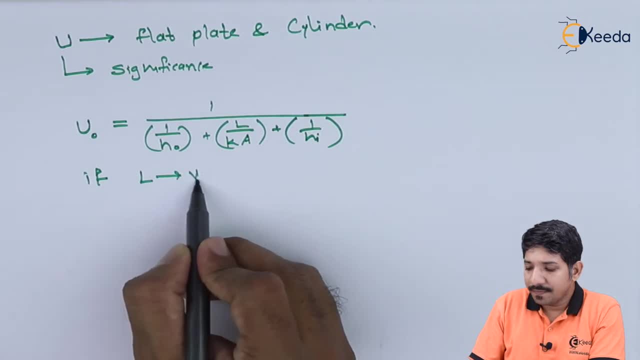 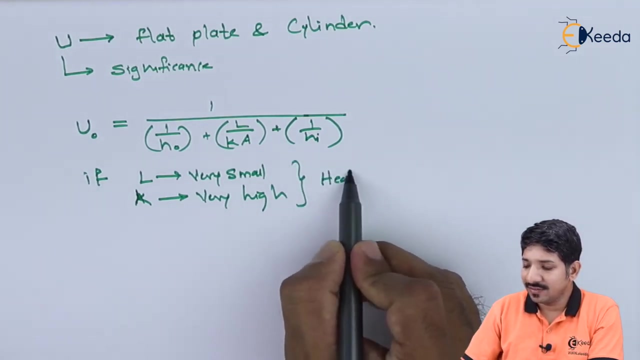 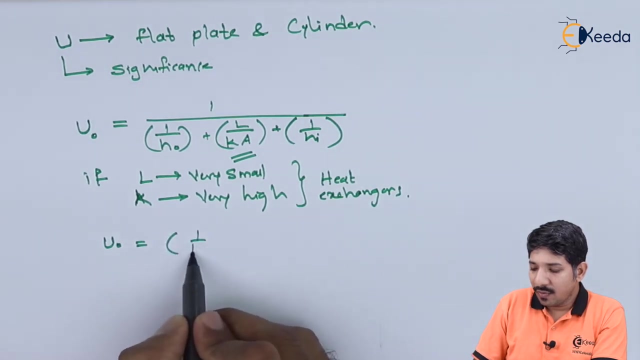 the l is very small. k value, thermal conductivity, is very high. If this is the case, so this case you will find in most of the heat exchangers. If this is the case, then we can obviously neglect this quantity. So we can easily find the value of u o as 1 upon h o plus 1 upon h i inverse. 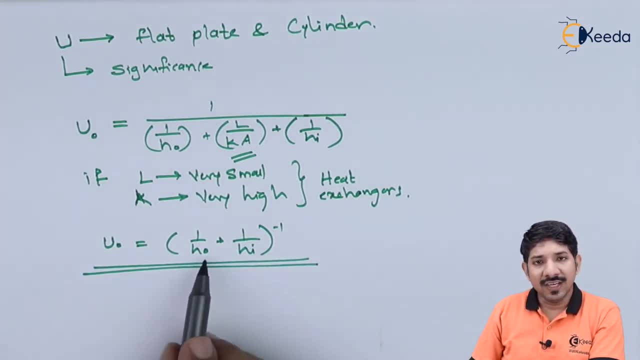 So this way, if I know the value of heat transfer coefficient for the 2 fluids, I can easily find out the overall heat transfer coefficient. Similarly, if suppose the one side we are having gas- Let us say this outside- indicates gas, Then we know the value of S0 is very small. 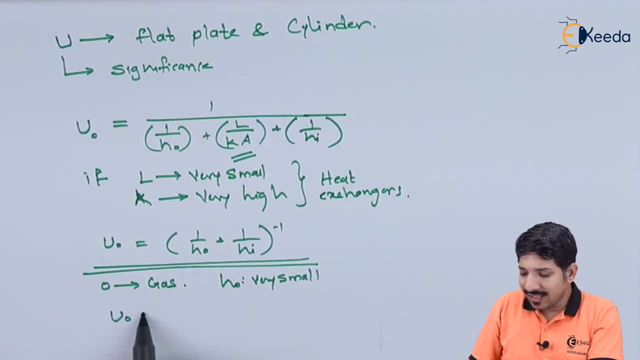 So we can neglect this quantity and the overall heat transfer coefficient can be easily found out. So this way, if I know, the value of h? o of s0 is very small, So we can easily be said as that of the, the heat transfer coefficient for the inlet fluid, such as liquid. 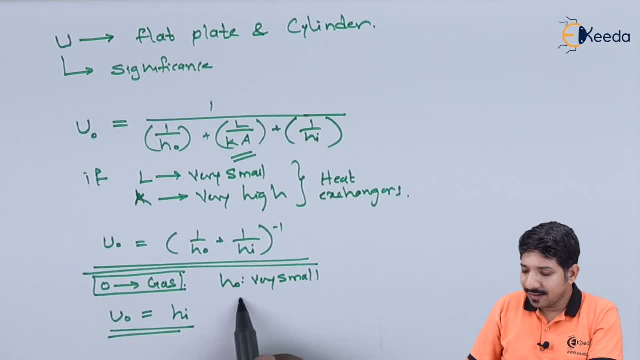 So in this case, we have assumed that O was gas and the I we have considered as liquid. See, if this is the scenario, then the overall heat transfer coefficient can be easily equated to the heat transfer coefficient of that of the inlet fluid. Now, in this case, what we do, we know.